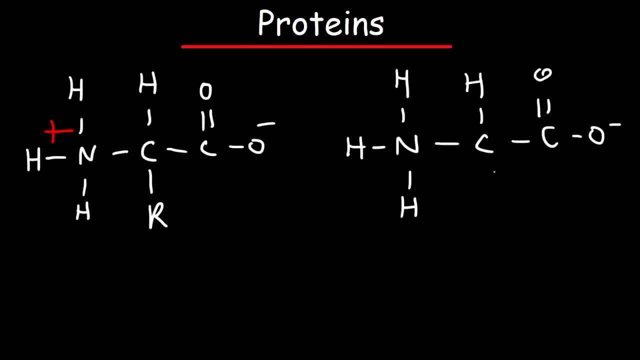 the carboxyl group is the C terminal of the amino acid. Now these two amino acids can react with each other in a condensation reaction. Now these two amino acids can react with each other in a condensation reaction, where we're going to lose water and we're going to connect the two amino 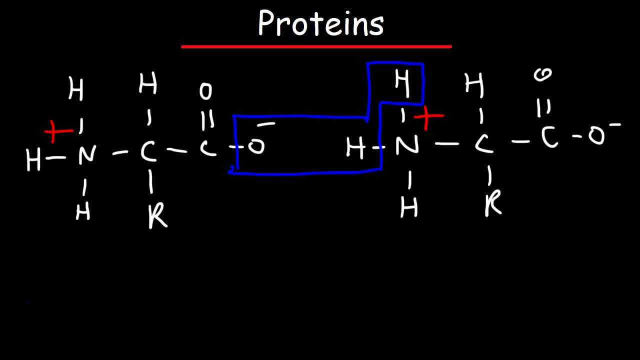 acids into one molecule. so once water is removed, we could form a peptide bond. this is also called a dehydration reaction, because you're losing water, and so this is going to be the new product of the reaction. So let's see if i can fit it in here. 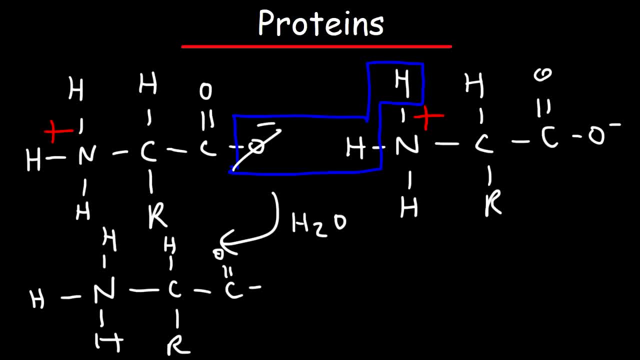 here. So this oxygen is gone. So now we have a nitrogen. Let me take out H2O. We have one hydrogen left over. We lost two once we lost water. So this is a dipeptide, because we have two amino acids combined And so this amide bond. 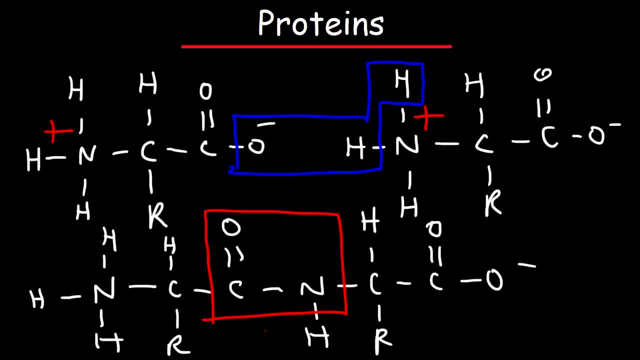 that we see here. that is the peptide bond. We formed a bond between the carbon and the nitrogen atom. So whenever you combine two amino acids to form a peptide bond, you're forming a covalent bond Which is hard to break. Now let's talk about the different levels of protein structure. 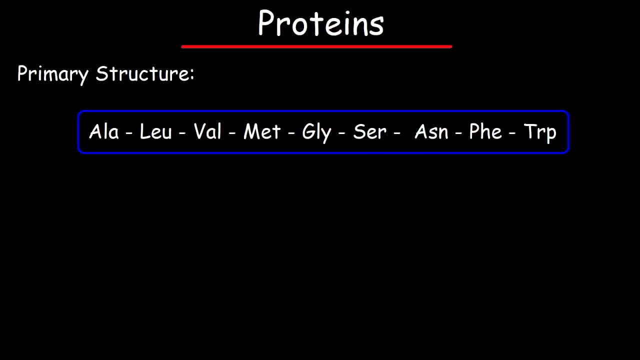 There's four levels that you need to know: The primary structure, the secondary structure, the tertiary structure and finally, the quaternary structure. Now, the primary structure is simply based on the sequence of the amino acids found in the protein. The sequence determines the shape of the protein If you replace the structure with the amino acids. 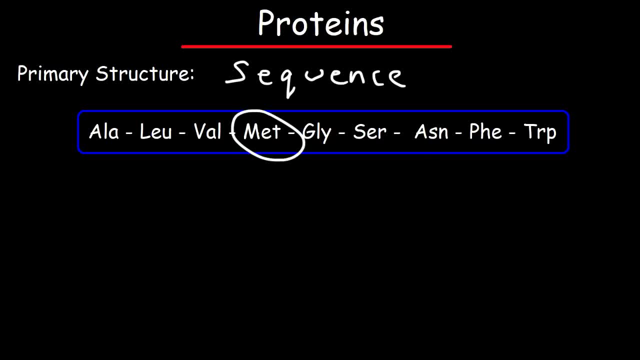 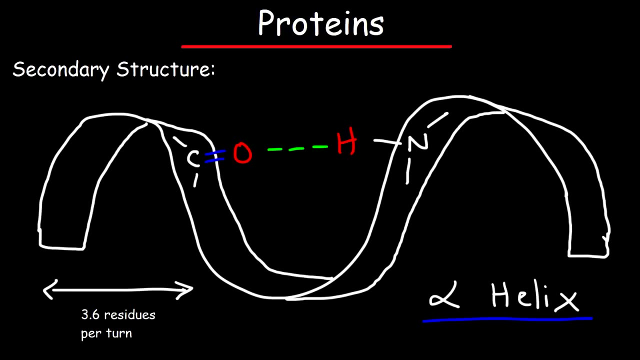 found in the protein. it will completely change the shape of the protein, So the shape and its function is primarily determined by the sequence of amino acids. The secondary structure describes the localized shape of a protein, And there's two of them that you need to be familiar with.